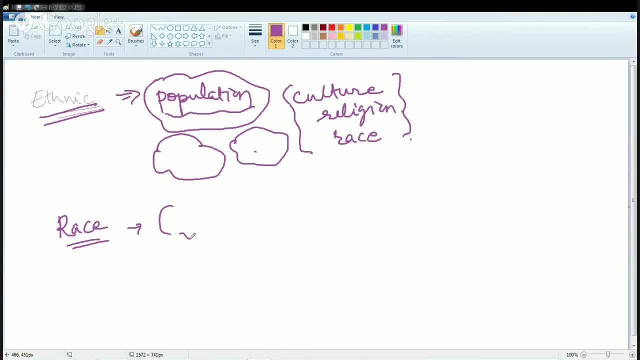 when i talk about race, i say it is a group of people sharing common genetic or biological ancestry. so here the main concept is: it's a biological inheritance and here it is a cultural inheritance. so this is the primary difference between the term ethnicity and race. most of the students get confused with this concept a lot. now there is a next term. 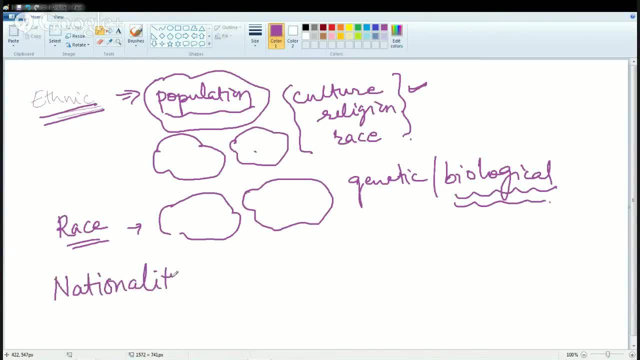 which is known as nationality. what is nationality if i say, if i belong to this ethnic group, which is a group of people sharing common genetic or biological heritage? i say it is a group of people sharing common genetic or biological heritage. i say it is a group of people sharing common genetic or biological heritage. i say it is a group of people sharing 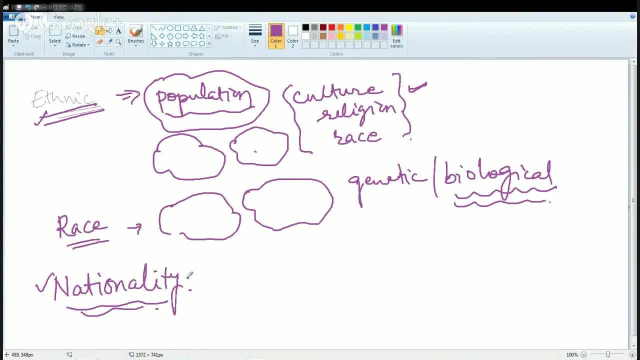 common genital offspring. I have nickname will always follow under nationality. people in channels are not necessarily Wyeth, is it? will i be a national authority? will I follow that nationality? Is it a correct statement? I can say it's definitely an incorrect statement, because nationality is a further different concept where I say it is an group of people. 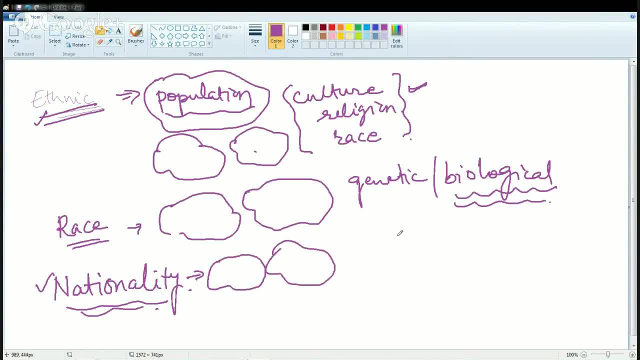 or a population That is sharing the common legal attachment. so if i am legally a fan to some country or some territory, that is what is nationality. What is nationality? So I have my personal ancestor or representant look like international thing or are unique people and direction. and to understand how bee this genital- here is71 column is, I am looking. 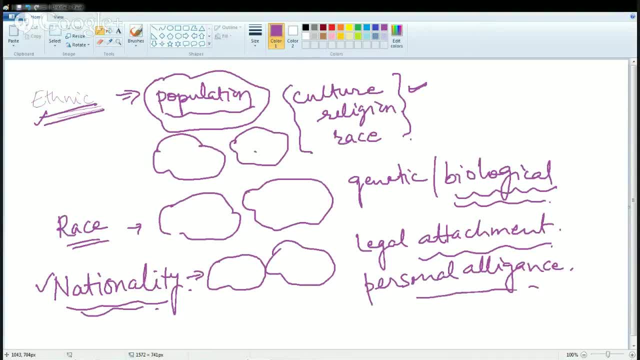 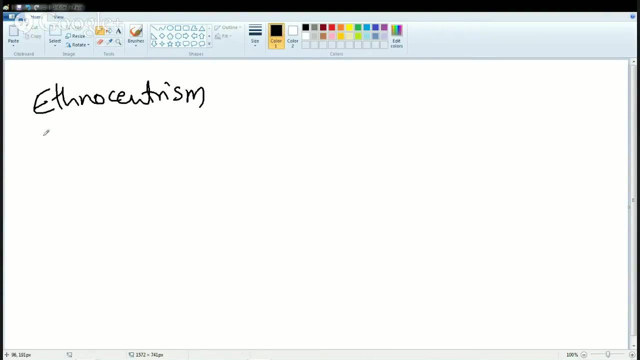 elegance to that country, and that is what is nationality. so this is the primary concept of ethnicity, race and nationality. now, before we go further into the concept of ethnicity, lets understand few primary terms that are related to the concept of ethnicity. the first is the concept of ethnocentrism. ethnocentrism is a concept mainly used in philosophical 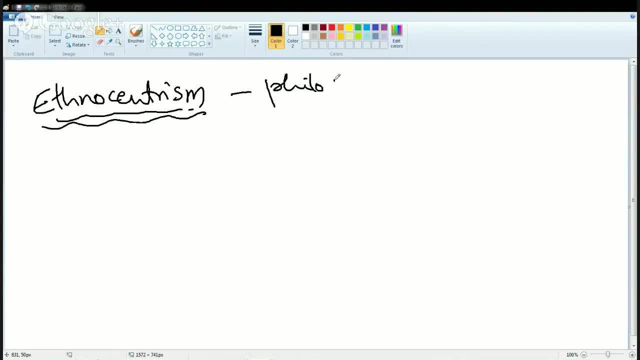 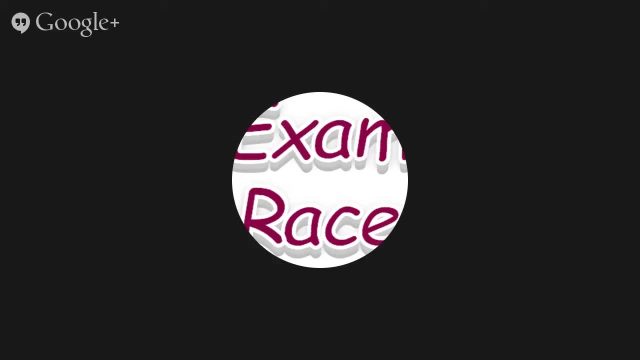 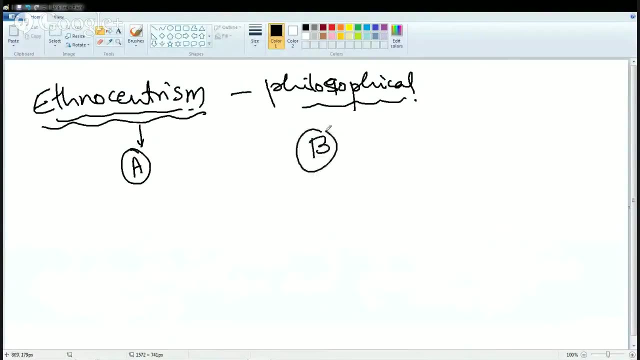 constructs and this concept talks about the separality when one believes about one's ethnic group. so if I belong to supposedly ethnic group A and one of my colleagues belong to ethnic group B, I believe in all cases the ethnic group A is superior to the group B. 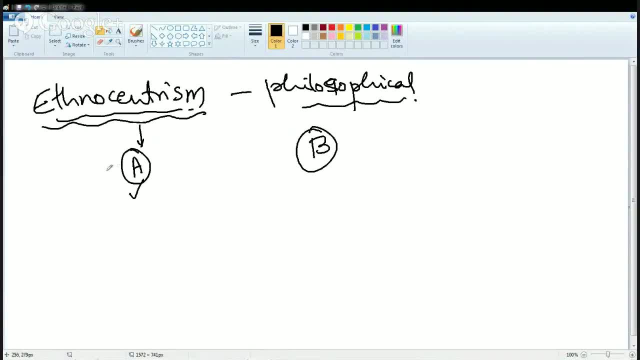 that means I am ethnocentric towards the ethnic population of person A based on this concept. so that is what is ethnocentrism: where I have a predominantly predominant belief that my group is superior to the another sect or another group of population. the next term we must know here is ethnic island. what does the word ethnic island? 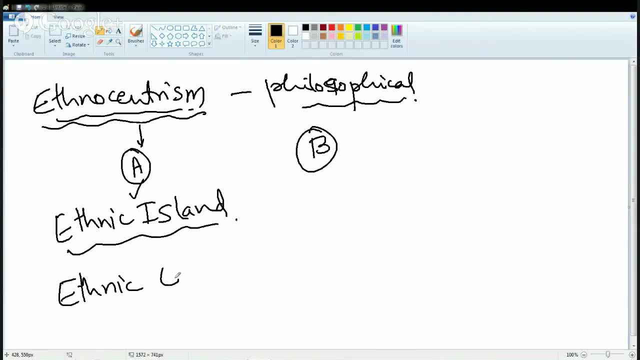 mean and how is it different from ethnic enclaves? there is a minor difference between the two, but there is definitely a significant difference because these two terms are not similar, which most of the candidates get confused with. so let us first understand what is ethnic island? so ethnic island is a. basically, I have a. 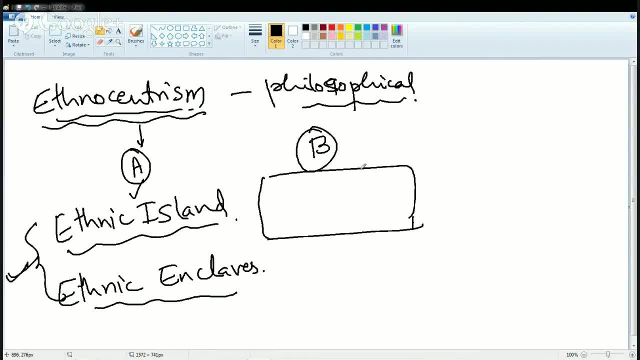 huge set of population here, since the whole city of New York or any big city, any big urban area, and within that urban area I have a minority cultural group and I have a minority cultural group and I have a minority cultural group which is distributed in the region and that is known as ethnic island. so the classic. example of ethnic islands are Germans located in south central Texas. that is the most popular ethnic island example we can do. and second is a lot of Scottish people from Scotland and Ireland, so Scottish Irish people, living in the Appalachian mountain zone. so these are the two classic examples of ethnic island. now let us understand the next. 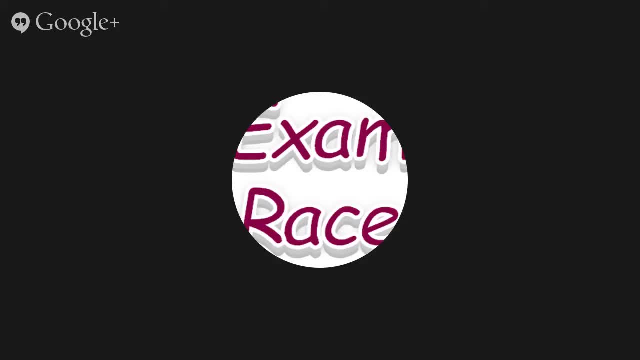 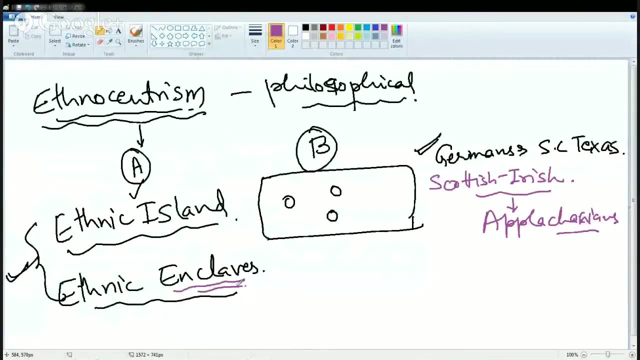 concept that is, ethnic enclave. what is enclave? so, when we talk about ethnic enclaves, it's a small area of the city that is inhabited by the minority group. for example, you must have heard of Chinatown. so what is Chinatown? Chinatown is predominantly a region dominated by Chinese people. 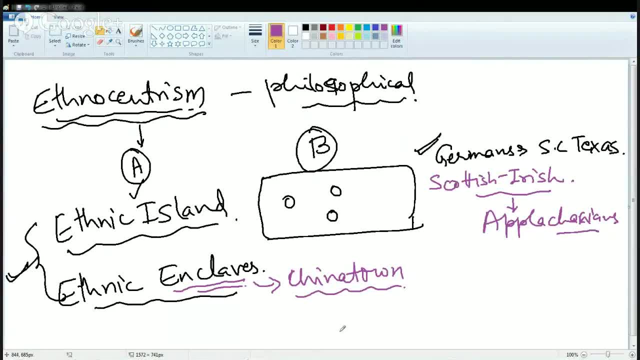 what is Chinatown? Chinatown is a meinem são um, myth tua um, and that is what is an among the villages in Tamil Nadu and in southern India, Yi, Baltimore, and in southern India, for example, all of these villages are pendants in number. now, in southern Malaysia, they are two groups of ethnic enclaves and we have happened, oh yeah, or what does it mean? within the city? so within the city, so like all the cities, most of the cities which have in the town, so that is what is an entity. So they try to preserve their identity or ethnicity in that region. similar is a military東 Telstra island. you become a ti town who have paul scriptures, and so they try to preserve a bay. well, the plunder. you have a little segment. so these are some examples of ethnic enclaves. now we are talking about ethnic and clearly Thailand. we have talked about ethnic encl conflict. so O Андachen und das spatula. so where is you know? we have talked. 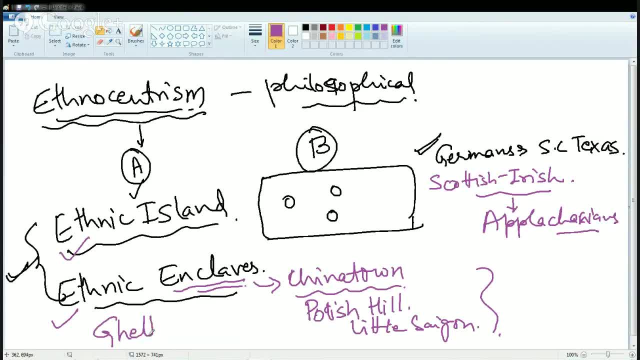 about ethnic islands. what is ghettos? that's a similar term you might have heard off and on, but what is ghetto? ghetto is a kind of ethnic enclave, but in ghettos people are usually forced to live in that region. so it can be of two types. 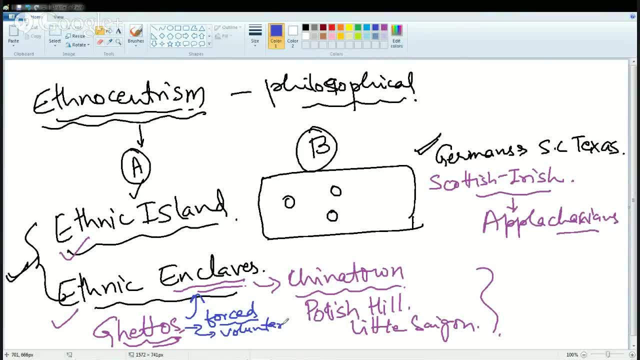 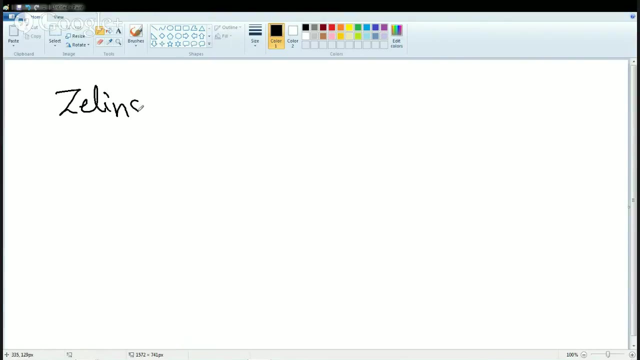 either they are forced or it is voluntary, but in either case it is a total segregation. and this ghettos are usually demarcated based on race or religion. this is the primary reason for demarcating any ghetto: is race or religion. now, there was a famous geographer who worked in this concept is Zelensky. 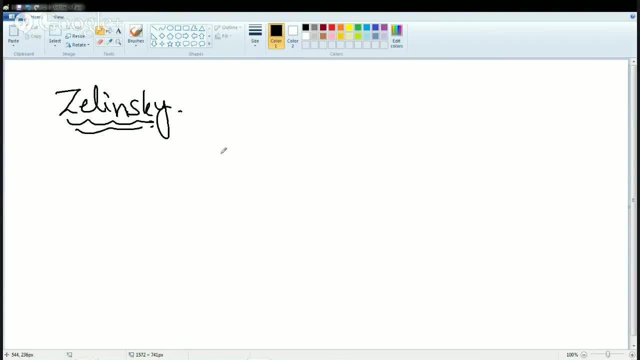 Zelensky said that whenever any ethnic group enters into a country or any new territory, it tries to establish a first effective settlement. that first effective settlement, I can say, is known as the Charter group or the Charter population, and this Charter population tries to establish the new concepts, new ideas and 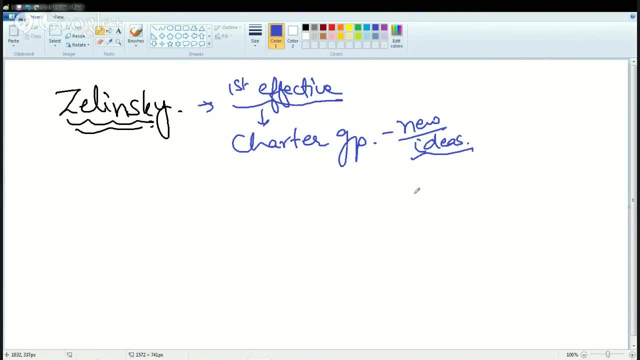 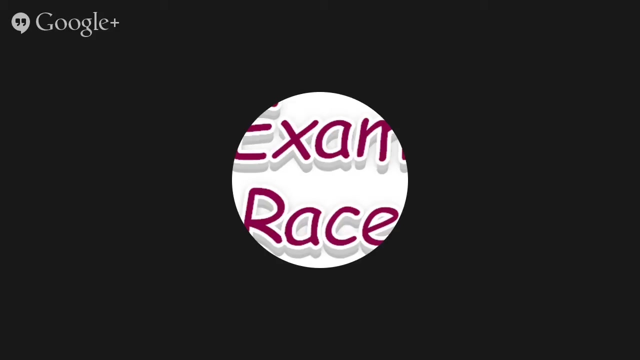 new philosophy of their ethnicity. so a classic example is when migration in US took place, which was basically predominantly by Native Americans. so when people from England, Ireland, Scotland- these were the first settlers in US, so people from England, Scotland and Ireland move into, what happened was this region was the first. 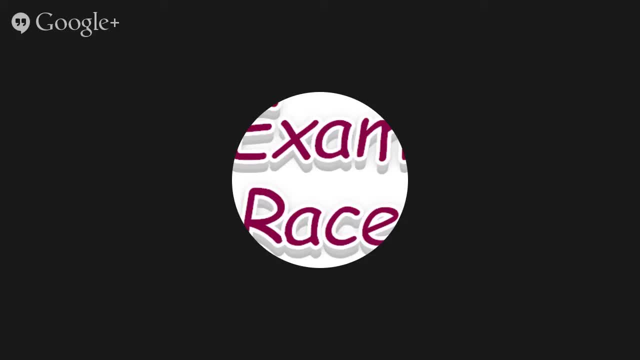 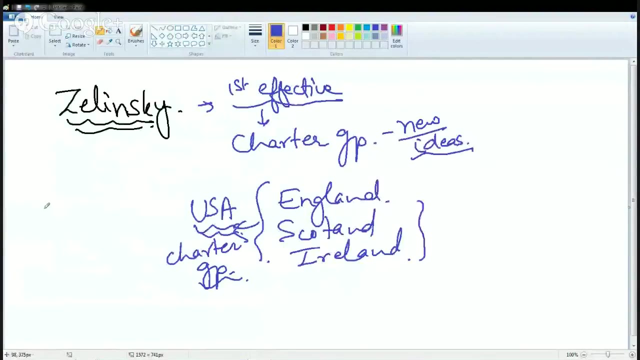 to be charter first, where the Charter group came to establish, and this concept was given by Zelensky. This concept was given by Zelensky is a very important concept to understand ethnicity now, when we talk about ethnicity, why ethnicities are demarcated and basically what happens based on demarcation. when I talk 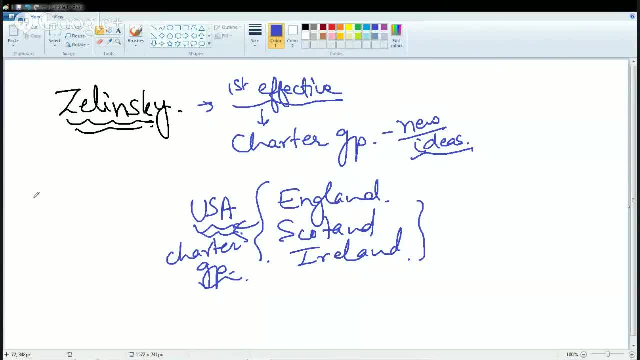 about ethnicity. what the predominant population does here is tries to clean it out. so if I am located in a city, a for example, what I will be doing is I will be trying to remove all other ethnicities from the region, and this phenomena is known as ethnic cleansing. 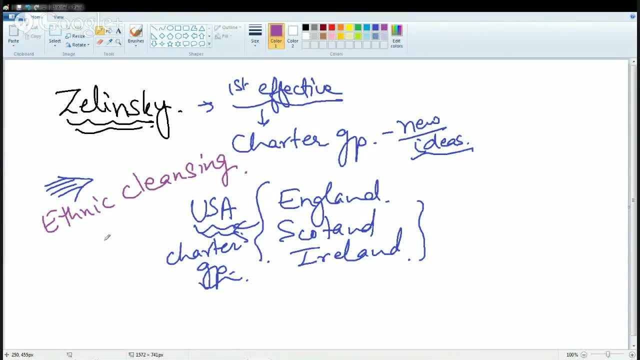 so ethnic cleansing is basically removing of one ethnic group by another group. so that is what is ethnic cleansing. now we talked about ethnic cleansing. now a similar concept is balkanization. balkanization is an important concept that is recently being used. now let's first understand the concept of balkanization. balkan states is a region. 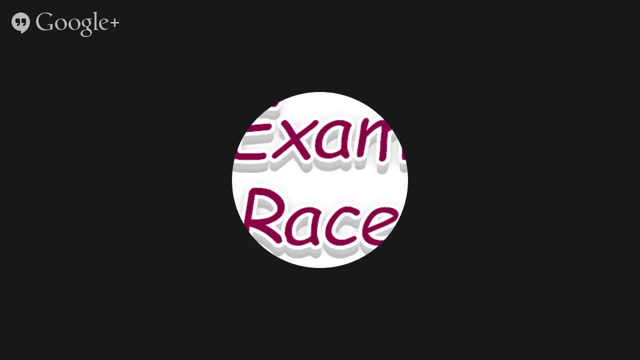 surrounding between Russia and Asia. so it's basically Russia, Europe and Asia. so this area is basically a small geographical area which was not able to organize. it was not able to organize due to instability in the region and due to a huge number of ethnic diversity. so what happened when the demarcation took place? what people did was they put all the 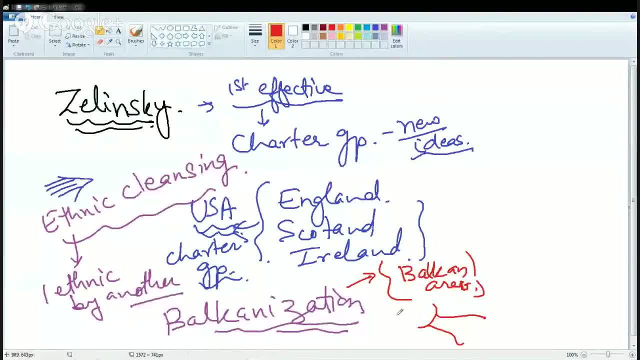 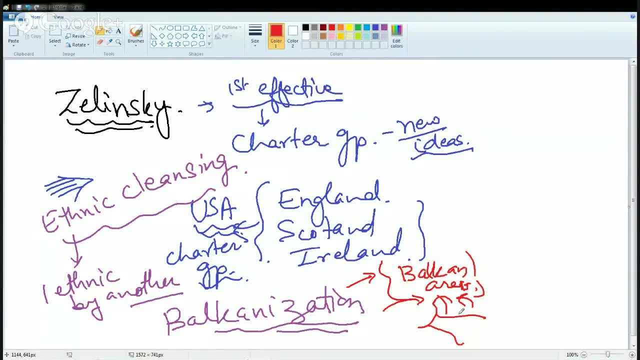 of a kind of a group of different ethnicity. there was a term, balkanization, which became popular, and wherever there was, there comes up a group of ethnic population which is which cannot lead to a stable state. we call it balkanization. so this term became popular. only after the first and the second world war balkan states became prominent. 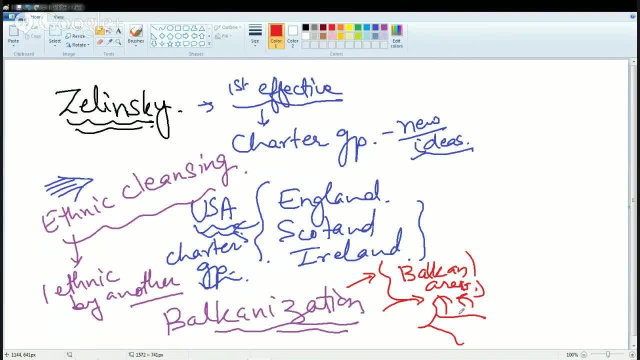 in South Russia. so next is the term that we need to understand is genocide. what is genocide? Genocide is basically a large scale killing of one ethnic group. Genocide became a major issue of concern during World War II, when Nazis attacked Jews and they tried to wipe 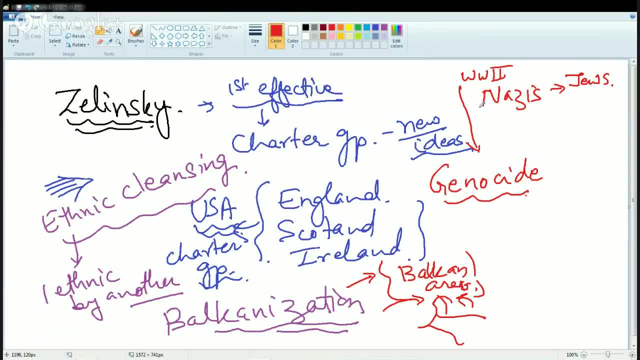 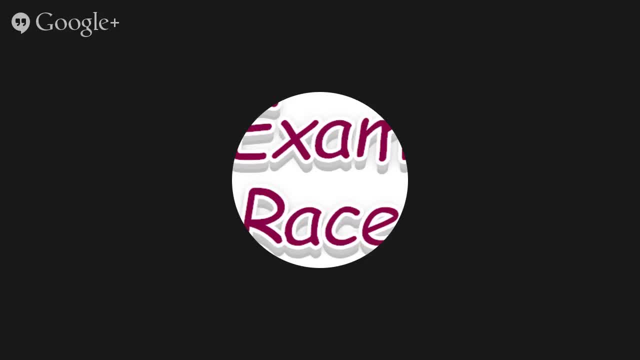 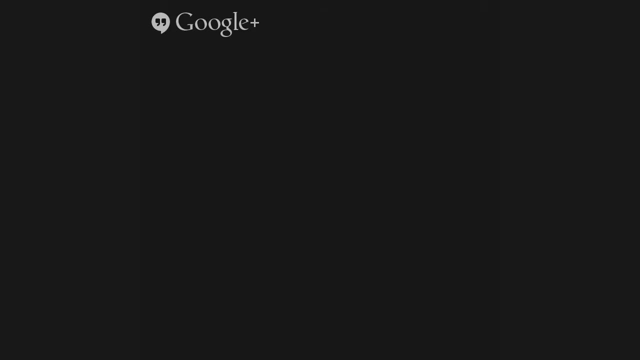 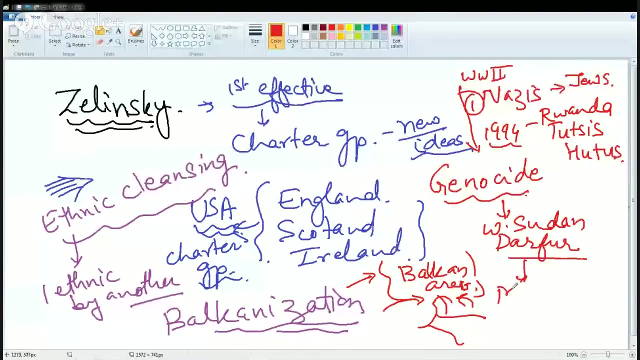 out the population of Jews. This was one of the important cases of Genocide. The other recent case is in 1994, there was a conflict in Rwanda, in Africa, between Tustis and Hutus. The next case was in the region of Darfur, Here a Muslim-dominated sect known as Janjaweel. 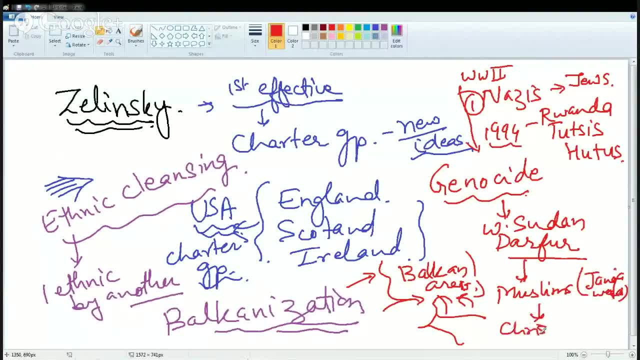 tried to eliminate all the Christians and Animists. Animists are the people who follow some objects. They consider any object of a specific kind and they try to preach those objects. So this is what is the difference between. this is what is Animist, So Western. 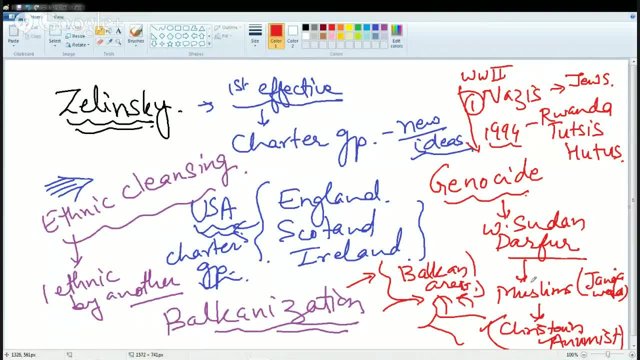 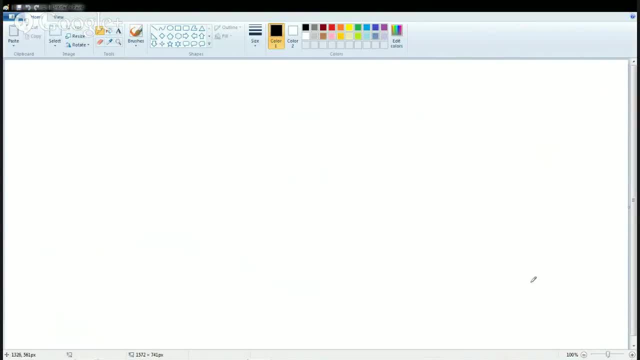 Sudan is another case of animism. Subtitles by the Amaraorg community: Genocide. Now we have talked about ethnicity, race nationalism. We need to understand where are the basic ethnicities located. So let's move out to the classic example of United. 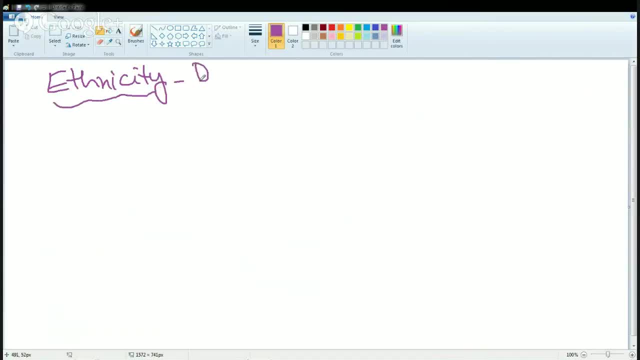 States of America to understand the distribution of ethnicity. If I classically talk about the distribution of ethnicity, I can say African-Americans contribute about 13% of their population, located mainly in the southeast states of Alabama, Georgia, then you have Louisiana, where the recent riots have been taking place, and then you have South Carolina. 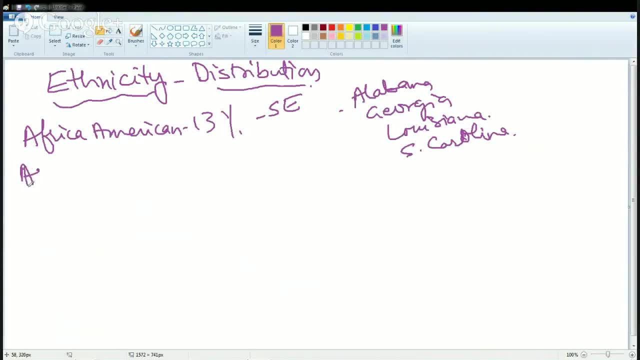 The next is the Hispanics or Latinos, which constitute 11%. So the Hispanic or Latino are two different, et cetera. And in the second case, the Hispanic or Latino are two different, et cetera. So the Hispanic or Latino are also considered 11% of the population. So 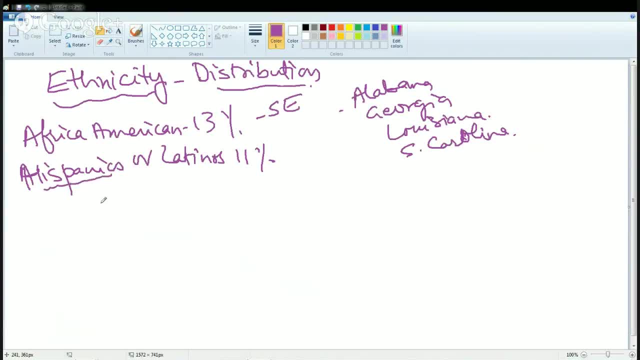 they all are talking about the racial and ethnicities. There's a link in the description. This is the problem that we have seen in term of discrimination, and it doesn't matter what the subcontractor's or the Spanish people speaking people mainly from Mexico are known as Hispanic, but later on. 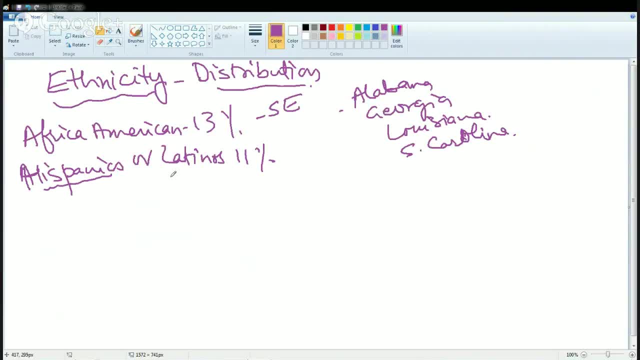 this term was considered as derogatory and now the term used officially in US as Latinos, which point out the Latin American population. So this contributed to about 11% of the total population in the United States, mainly attributed in the south west regions of California and Texas, pre-dominantly California and Texas. 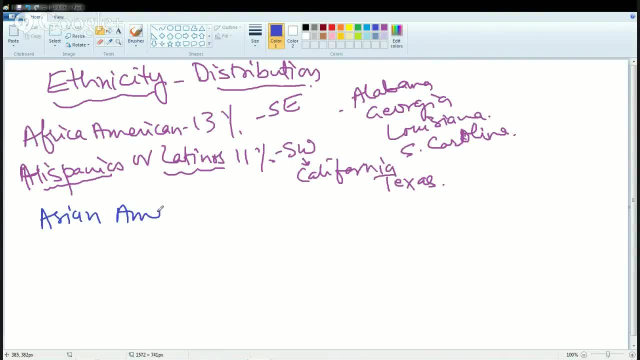 then you have the Asian Americans. Asian Americans contribute to around 4%, mainly located in the western regions. of these 4%, I can classify 25% as Chinese, 20% as Filipinos and 20% as Latinos, and the remaining 12% as Japanese or Vietnamese. 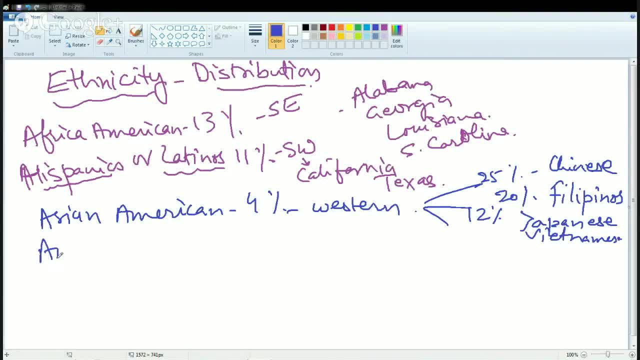 The next sect of ethnic population is the American Indians, contributing to merely 1% of the total population, mainly located in the south west region and the plains. Now, there is a difference. when there is an ethnic group that we are talking about, there are various ethnic groups. 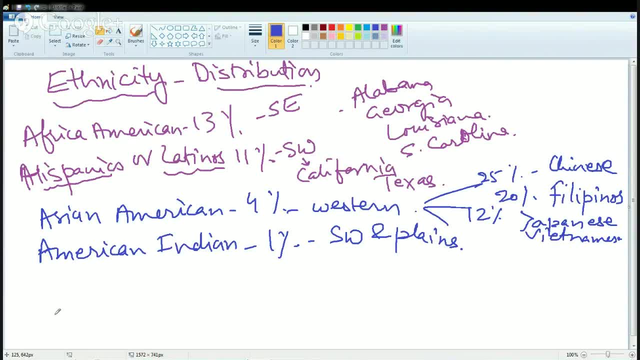 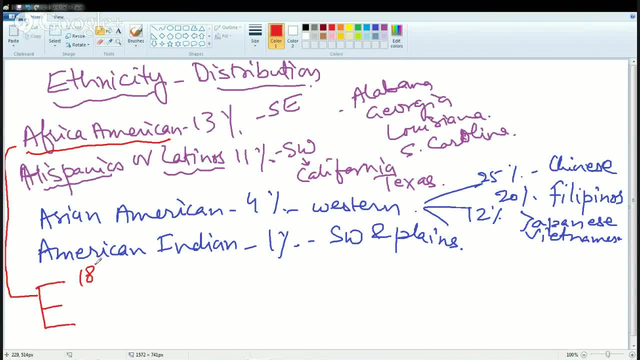 And this go back to the States of America today and that's the origin of the first teenagers coming to Western Canada And this access- we know that was actually to upstate cocain absorbed. the rate of the stage was migration to the north, As we can see, I said, African Americans are mainly concentrated. 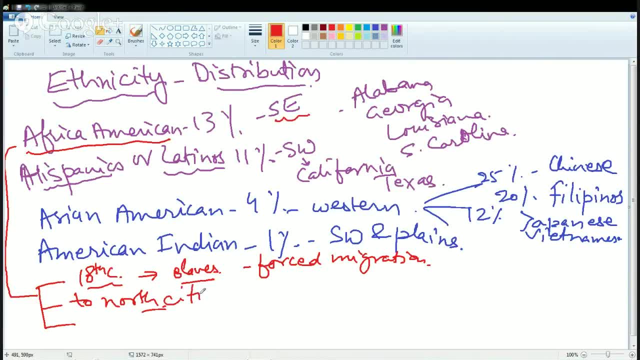 in the southeast regions. So what they tried to do was they slowly tried to migrate to the northern cities in search of jobs and other opportunities, And this became a prominent factor in the first half of the 20th century. And finally, what happened was there was a 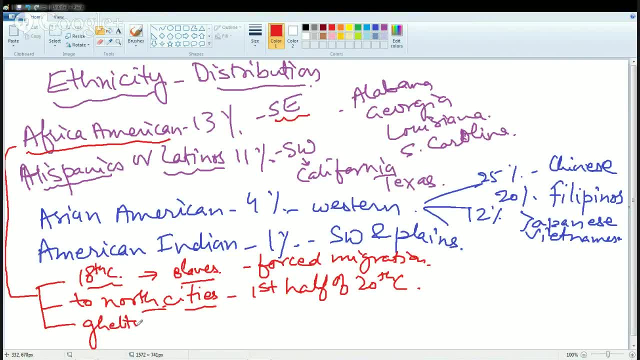 further migration from ghettos- what we understood recently- to the urban centers, And this migration is a kind of very recent phenomena and it took place in the second half of the 20th century. So these are the main. here we can understand the distribution of ethnicities and how they. 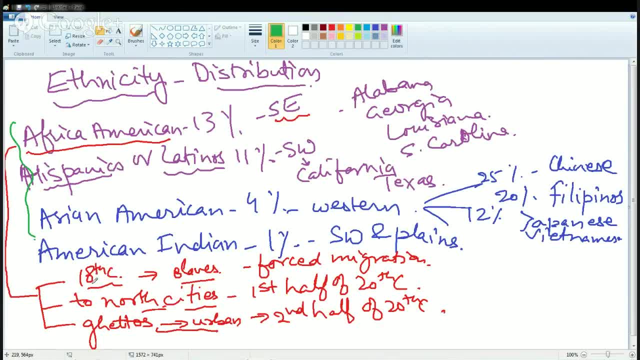 usually migrated and moved into the country. Now, which we will see in a little bit, is that for the earlier the process of migration they took quite a large period, But the first half of the 20th century it was 2,000 plus. 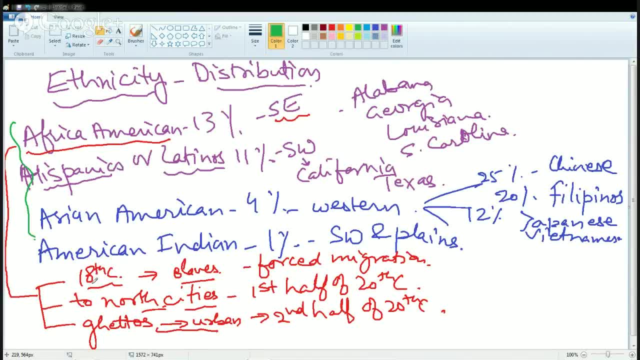 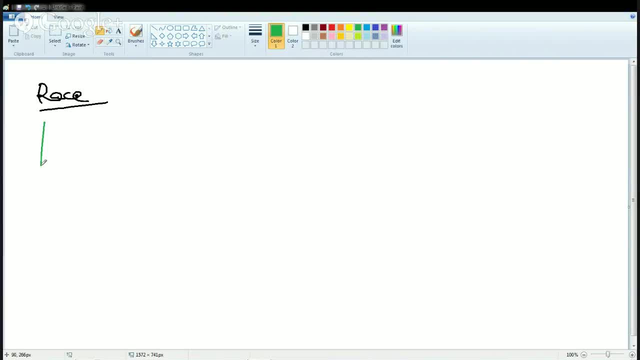 years, So the first half of the 20th century. they taken care of a lot of the migration. We talked about race, so we'll be discussing what is race. so race, as we know, is broadly classified into Mongolites, Caucasians and Austrians. but I'm not talking about the classification. 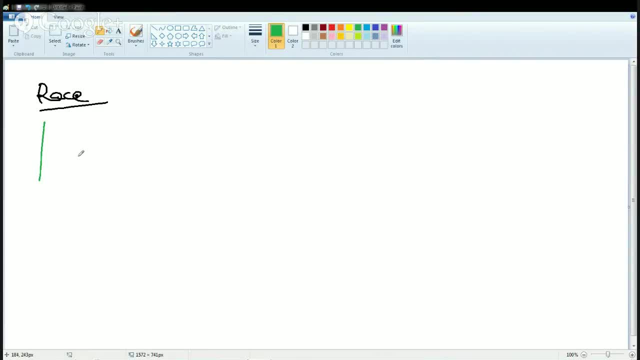 here. What we are trying to understand is the discriminations based on races. So the discrimination based on races, what is known as racism. there were various laws and doctrines that were incorporated, So the first was separate but equal doctrine. what does it stand for? 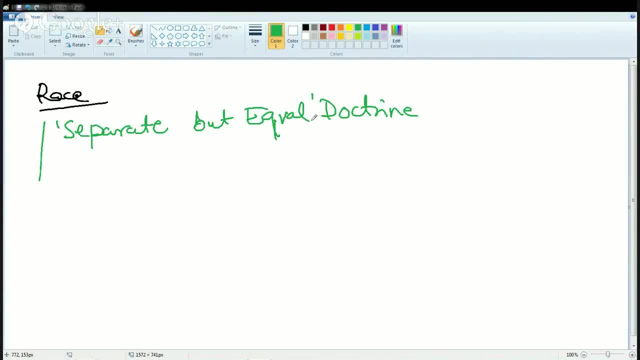 Separate but equal doctrine talks about giving equal opportunities to blacks and whites, but separately. So, for example, if there is a train running blacks and whites, there would be a different train, but you would be providing train to both, But there would be different train for whites and different train for blacks. 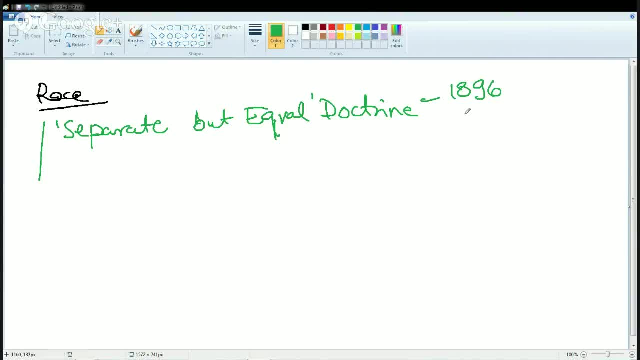 This doctrine was laid down by United States in 1896 and the Supreme Court of United States gave this decision under the Plessy versus Ferguson case. Later on, what happened was, slowly and gradually, this doctrine was abolished. from the system Similar to this doctrine, there was a constitution. 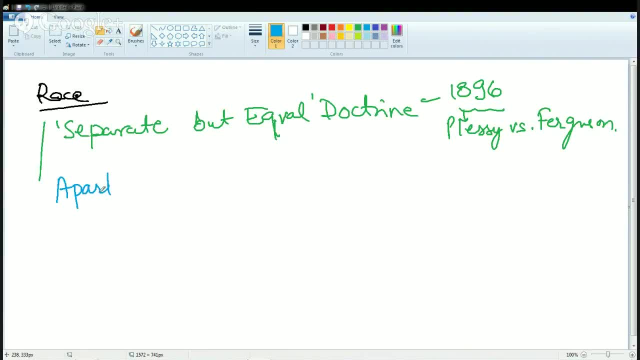 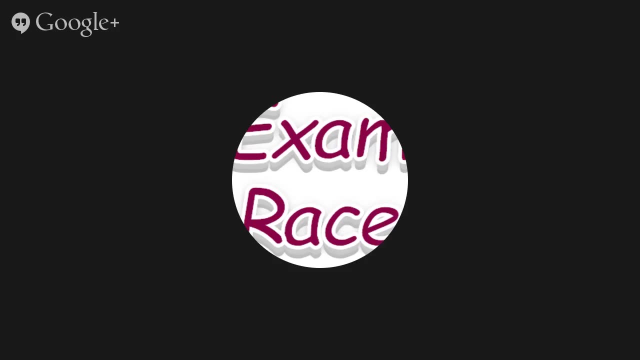 There was a constitution. There was a constitution. There was a concept of apartheid that is the most common and most heard of. So it was basically physical separation of races. So Nelson Mandela was one of the main person in South Africa who fought apartheid.